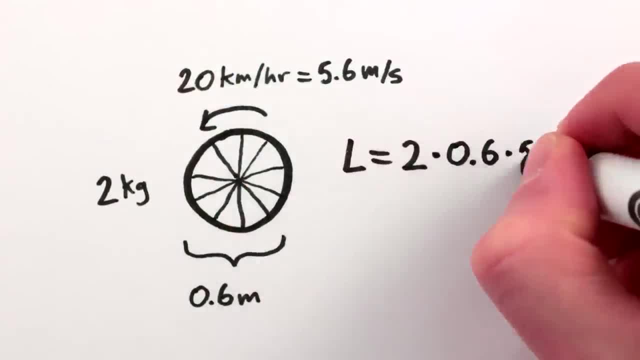 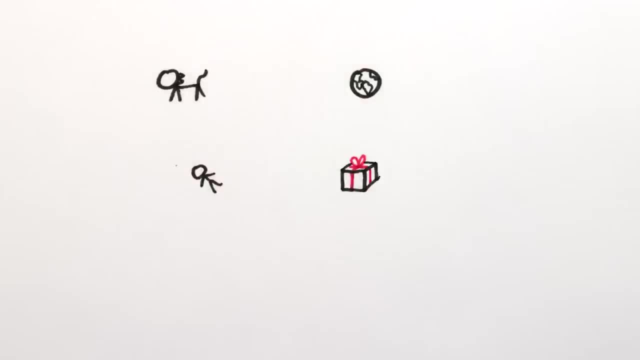 bicycle wheel going 20 kilometers per hour would have an angular momentum of about 7 kilogram meters squared per second. Is that useful to know? The reason we care about angular momentum is that if you take a bunch of objects that are interacting electromagnetically or 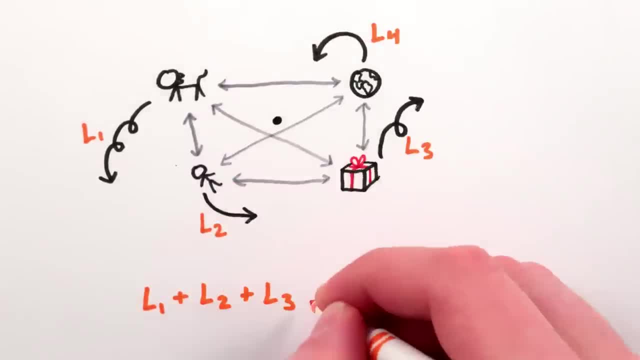 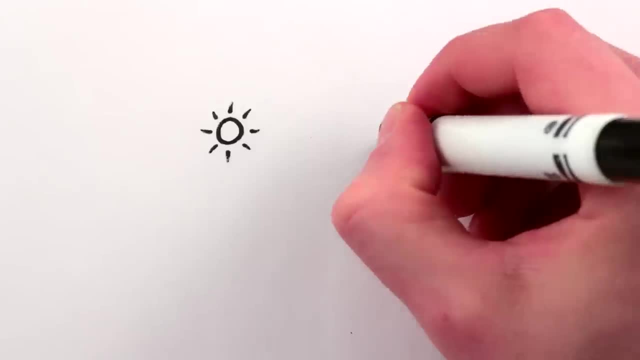 gravitationally or whatever, and add up all of their angular momenta into one number, then that total value won't change over time, Unless some other objects from outside come in and mess things up. So, as another example, the earth, which is 150 million kilometers from the sun, orbits. 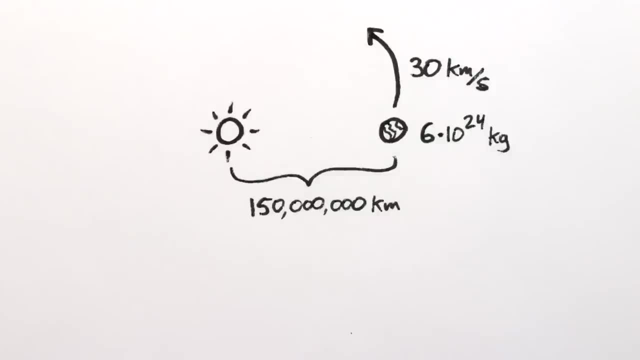 at 30 kilometers per second and has a mass of 6 times 10 to the 24th kilograms. has an angular momentum of 2.7 times 10 to the 40th kilogram. meters squared per second. That's 4000 quintillion quintillion bicycle wheels, And this angular momentum stays roughly constant. 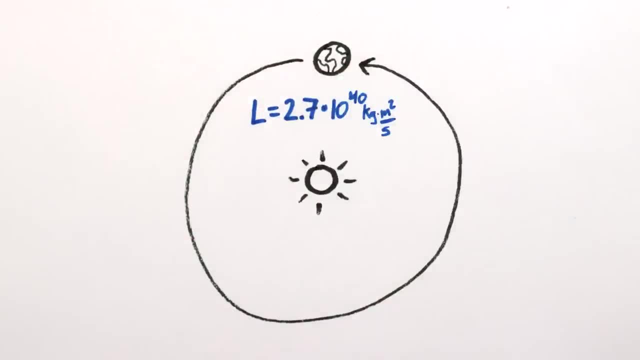 over the course of the earth's orbit, year in and year out. But what's amazing is that even if the sun and the rest of the solar system were to suddenly disappear, the earth would still have that same angular momentum about the point where the sun was. 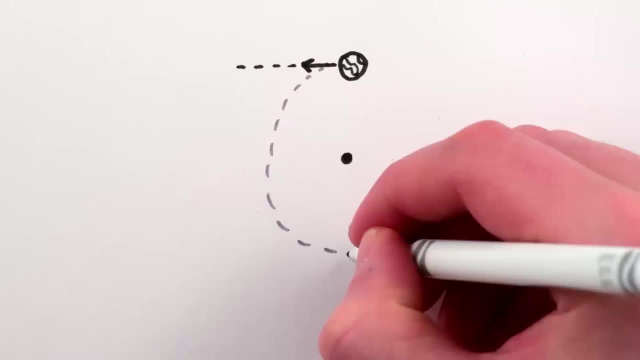 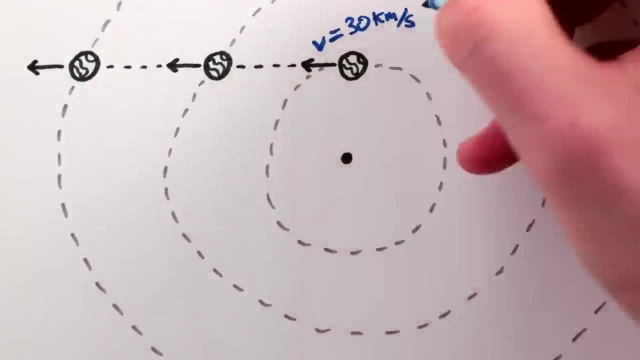 Without the sun's gravity, the earth would of course now move in a straight line, requiring an ever larger imaginary circle as it got farther from the point where the sun used to be. But as the earth continued through space, its 30 kilometer per second velocity. 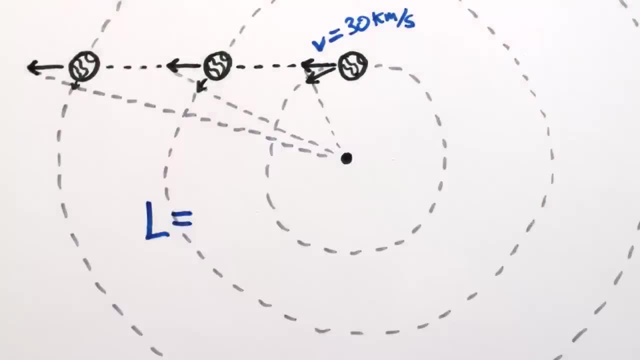 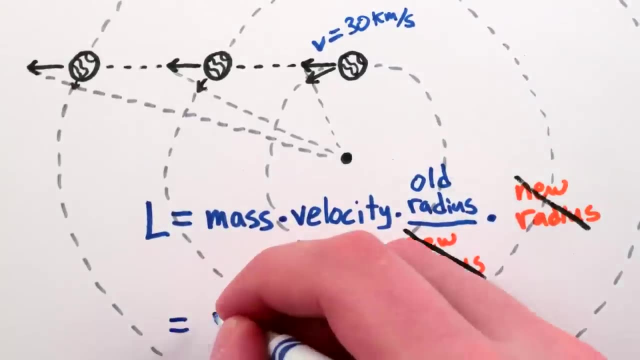 would also point less and less along the circle. so when you calculated the angular momentum, the decrease in velocity would exactly cancel out the increase in the size of the circle, and you'd always get the same answer: 2.7 times 10 to the 40th kilogram meters squared per second. 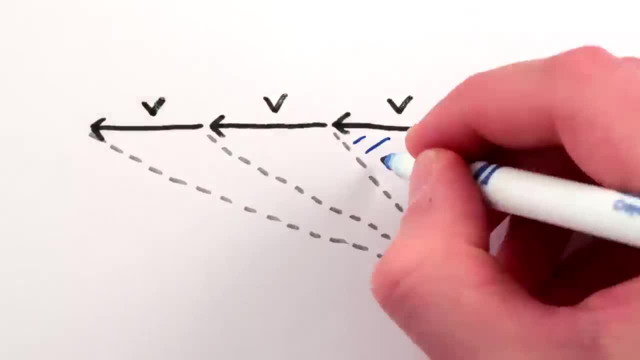 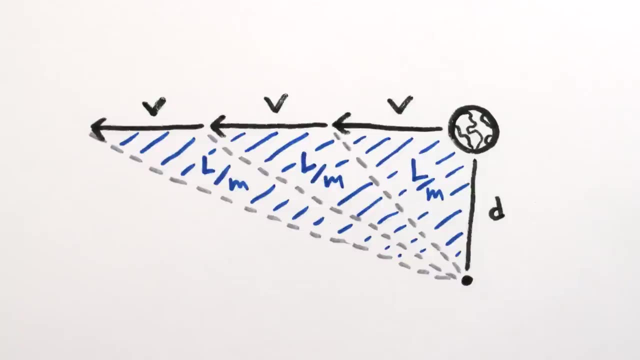 So, even when nothing is rotating at all, angular momentum is still conserved, And that's the beauty of a law of physics: It works even when you try to break it. This video is brought to you in part by Audiblecom, the leading provider of audiobooks across. 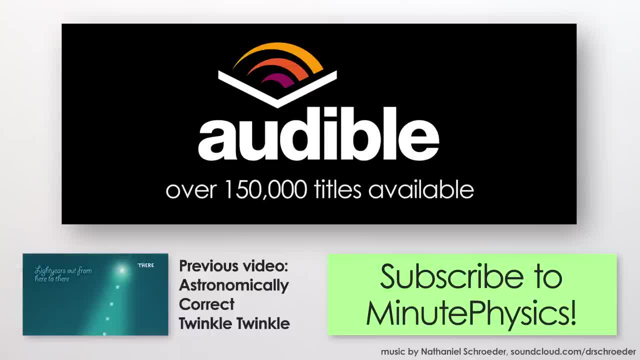 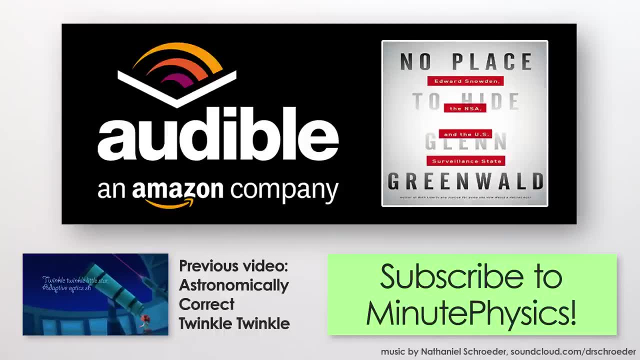 all types of literature, including fiction, non-fiction and periodicals. If you go to audiblecom slash minutephysics, you can try Audible out by downloading a free audiobook of your choice. I just read: No Place to Hide Edward Snowden, the NSA and the US Surveillance. 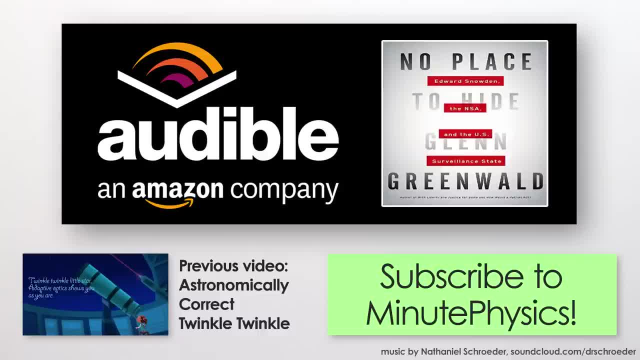 State by Glenn Greenwald, And I cannot recommend it enough. If you care about freedom or privacy or democracy and live anywhere in the world, you need to read this book Now, Again, you can download your free audiobook at audiblecom. slash minutephysics- and thanks to Audible for helping me continue. to make these videos.